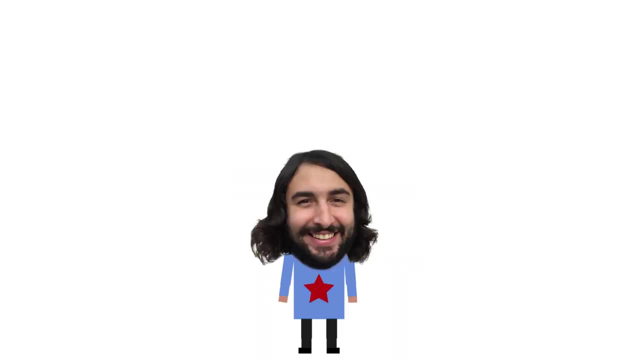 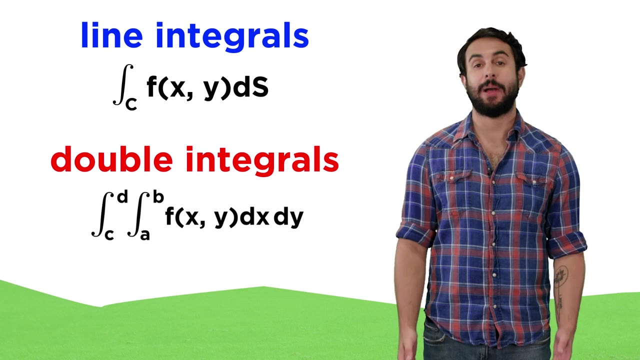 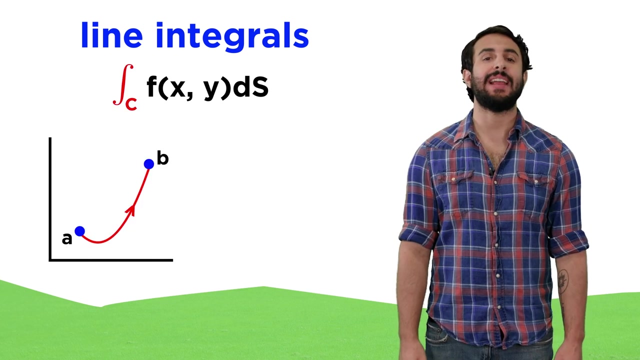 Professor Dave, here let's check out Green's Theorem. Now that we know about line integrals and double integrals, we are ready to learn an interesting theorem. Recall that with line integrals we can integrate along a curve C and if we have a vector field, 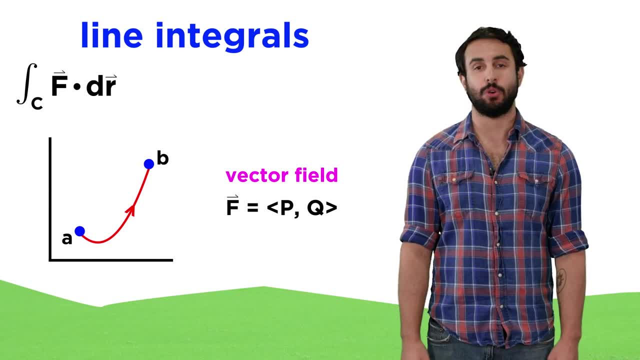 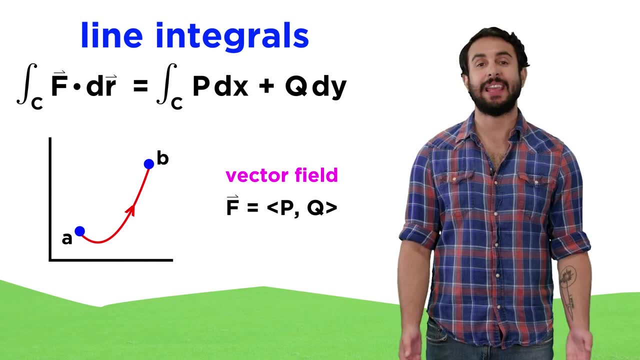 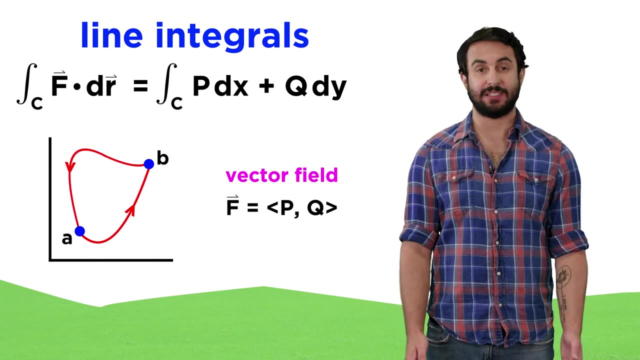 F equals PQ, then the form of the line integral is the integral along C of F, dot dr, which becomes the integral along C of Pdx plus Qdy. This is the case for all curves C. However, a special theorem exists for closed curves. 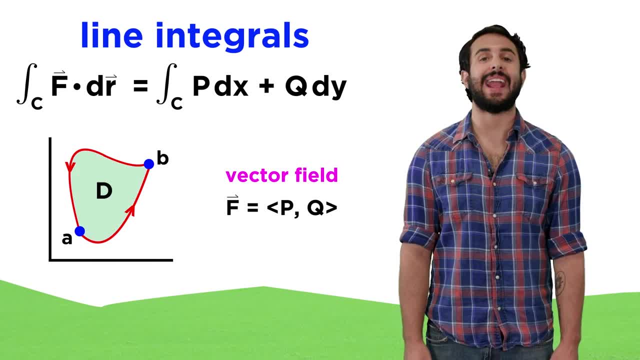 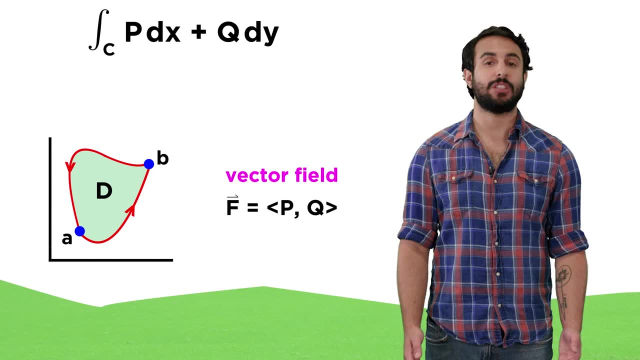 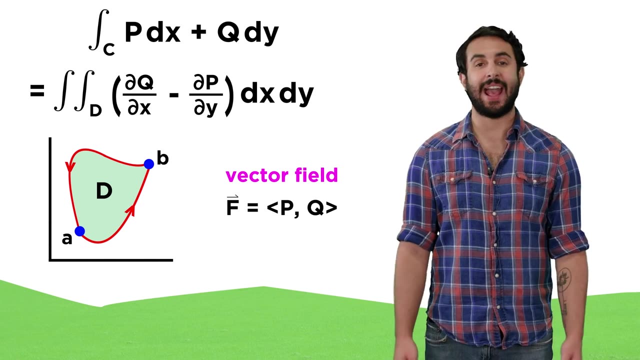 that is, curves that form a complete loop and enclose an area which we will label D. For these cases, the line integral over C of Pdx plus Qdy is the integral along C of Pdx plus Qdy, ends up being equal to the double integral over the domain D of dQdx minus dPdy. 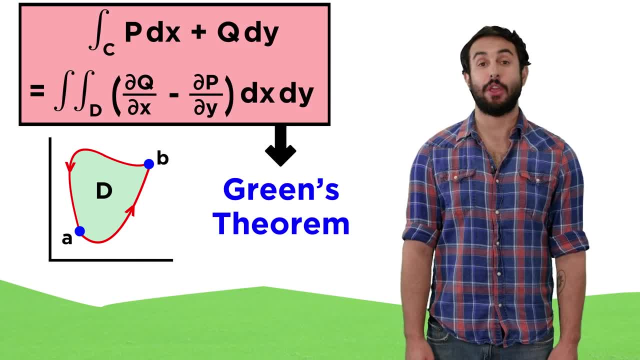 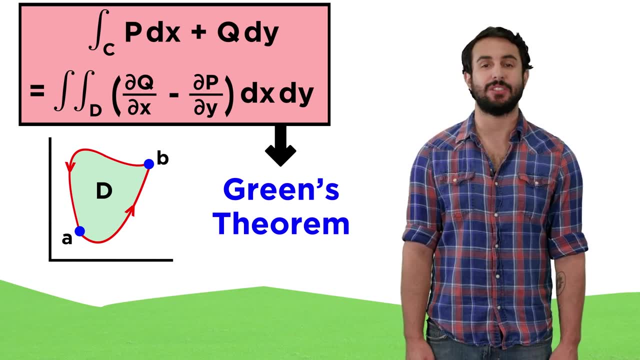 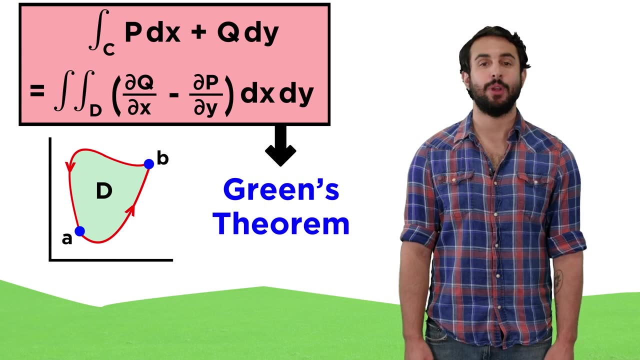 dxdy. This is called Green's Theorem. This is a very useful theorem, as line integrals are typically harder or more complicated to calculate than ordinary integrals, so this gives us a more convenient way to calculate them for closed curves. 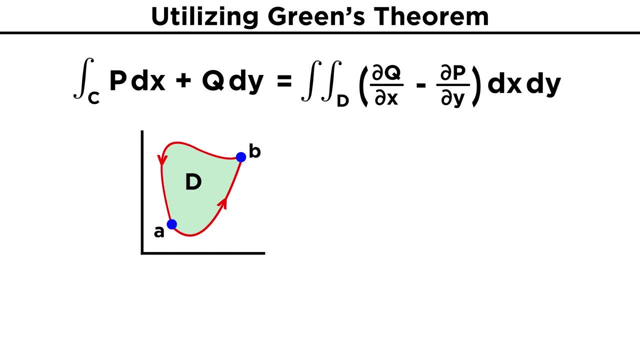 Before we move on to an example, there's an important distinction we must make regarding the direction of the curve. Green's theorem applies to closed curves that run counterclockwise. Another way to think of it is if you walked along the path in the direction of the arrows. 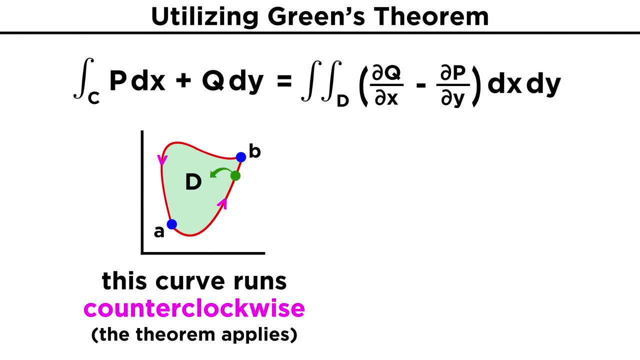 the enclosed domain will always be on your left. This is referred to as positive orientation For curves that go in a clockwise direction. the closed domain will always be on your left For curves that go in a clockwise direction, or negative orientation- Green's theorem. 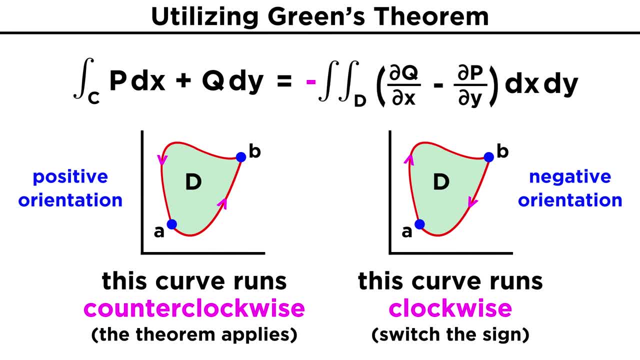 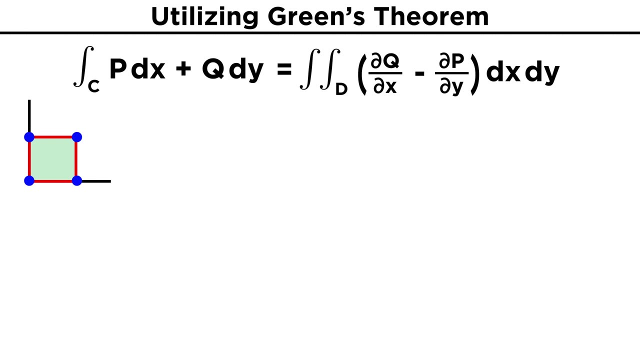 can still be applied, but with a sign change. so the line integral can still be expressed as a double integral, just with a negative sign right here out front. It will be important to remember this detail to get correct answers Now. for an example, let's say we have the curve shown here made of four line segments. 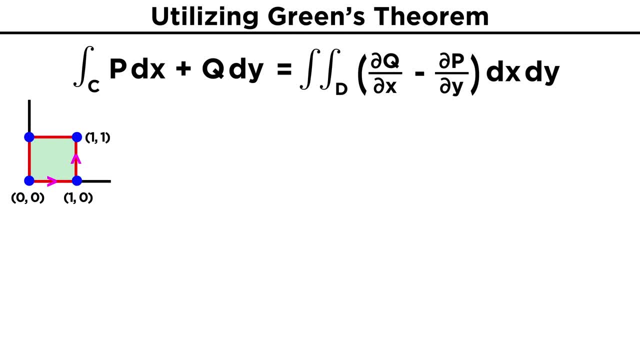 that make a square from zero-zero to one-zero to one-one to zero-one and back to the origin. We also have a vector field- F equals xy, x squared, and we want to find the line integral over C of F dot dr. 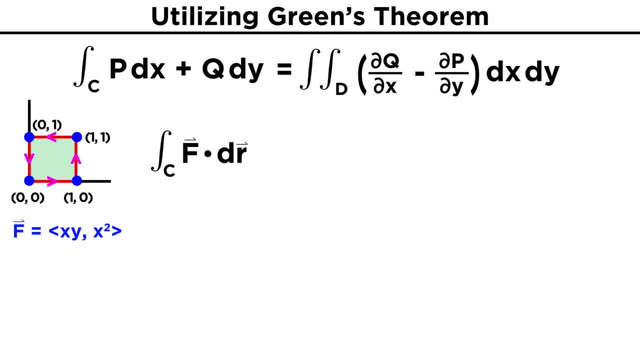 We could split the curve into the four line segments and do each line integral individually, but using Green's theorem can give us a much faster and simpler calculation. Our integration domain D ends up simply being a square where x and y both run from zero to one, so we have a double integral over this region of dqdx minus dpdy, dxdy. 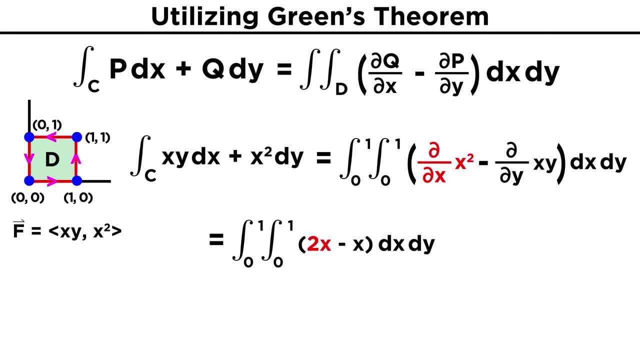 Our Q here is x squared, so dqdx is two x. Our P is xy, so dpdy is x. So we have a double integral over this region of dqdx minus dpdy dxdy. Our Q here is x squared, so dqdx is two x. 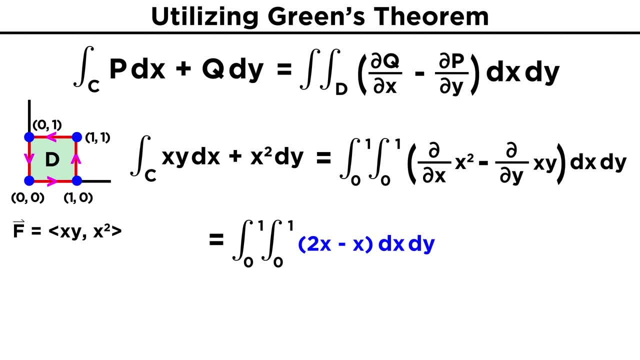 So again we get the double integral of two x minus x dxdy or just x dxdy Integrating x first, we get x squared over two, evaluated from zero to one, which gives one squared over two minus zero or just one half. 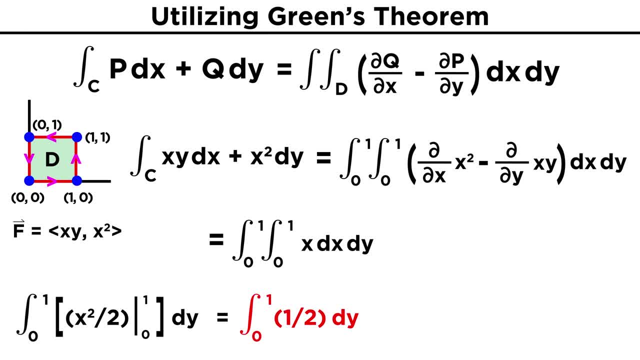 We still have the y integral to evaluate, but there's no y dependence left. we just have a constant Integrating. one half dy gives y over two, evaluated from zero to one, which just gives one half minus zero or one half. 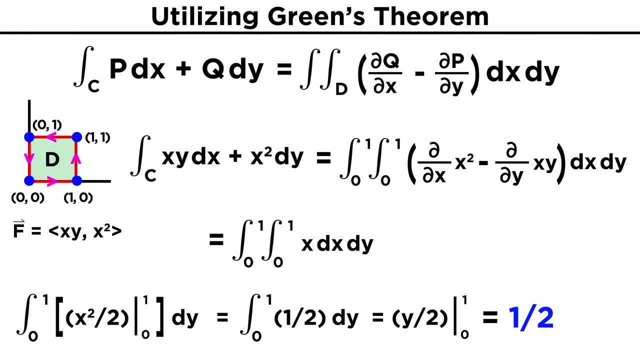 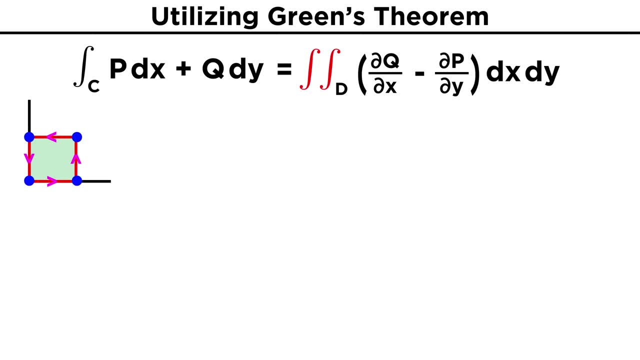 This is the value of our line integral. As you can see, Green's theorem gives us a much simpler method for evaluating line integrals on closed curves. Of course, not every boundary will be so simple to express. We will have to use the same kind of thought process. 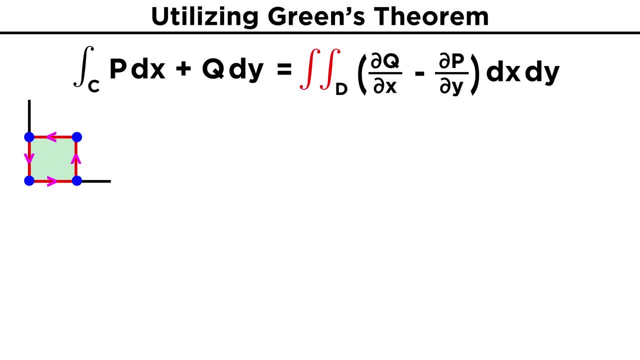 Just in the tutorial on double integrals to properly write the bounds of integration. For a quick look at this, consider the curve C given here, where three line segments make a triangle. The line segments are a straight line from zero- zero to one zero. from one zero to one.